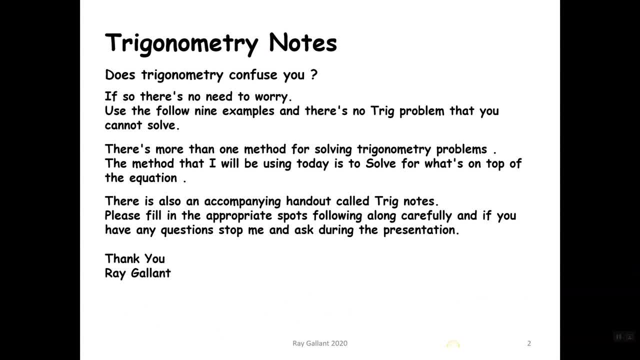 Some of the problems that we run into when people are trying to explain trigonometry is they'll take three or four different ways of getting there. Could you imagine trying to get to a store and then, every time someone shows you how to get to that store, they tell you a? 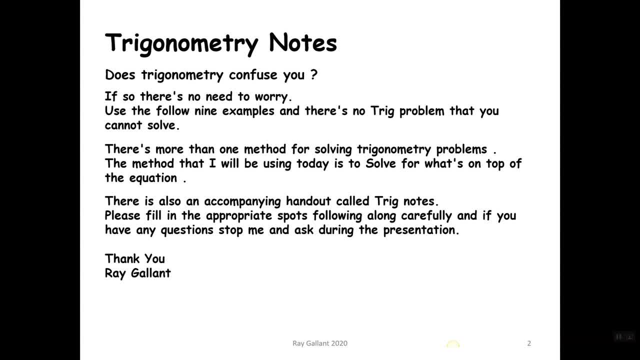 different way to get there. So I'm going to take a different approach and I'm going to show you how to get to the store- the exact same way every time. So I'm going to take a different approach and I'm going to show you how to get to the store- the exact same way every time. So bear with me Before we start. 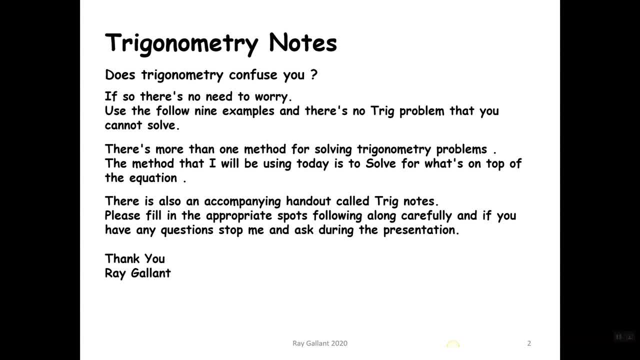 please go into the description below and download the file and have your calculator ready so you can go along with me while I'm doing these nine questions. By the way, there's really only nine trigonometry questions to solve all of your basic trigonometry problems. Okay, let's get started. 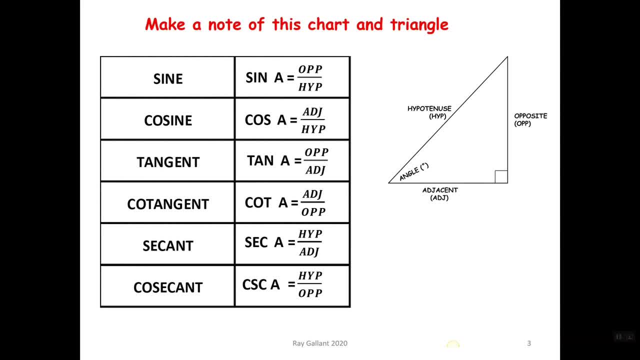 Before we start- and I shouldn't say before, because we're starting right now- we want to talk about the triangle. Okay, so if my angle's right here, the length or side that's closest to it is going to be the adjacent side. 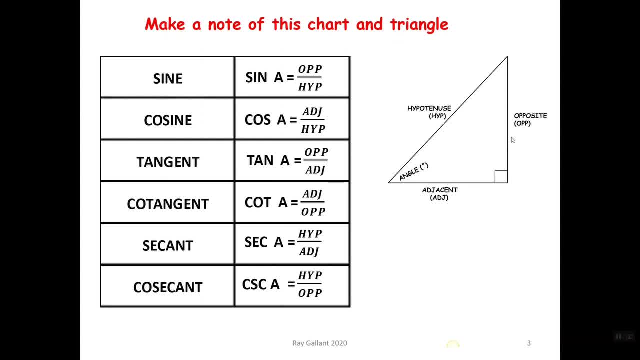 If the angle's here, the one that's furthest away is going to be the opposite side, And the part of your triangle that's the longest is going to be called the hypotenuse. So bear with me, we're going to test this theory out, If this is my angle up top here. 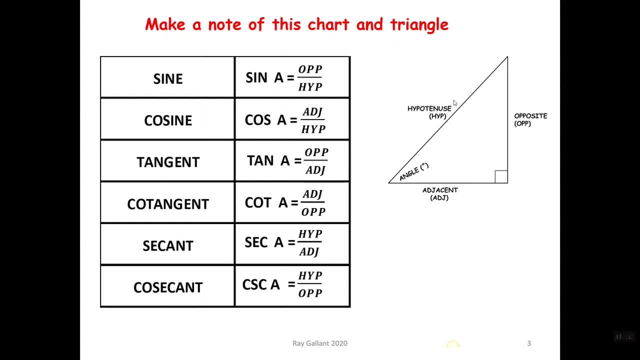 this guy here is going to be my opposite, my adjacent, and the hypotenuse, and the hypotenuse stays the same. Okay, let's take a look at our chart. here We have sine cosine, tangent, cotangent, secant and cosecant. 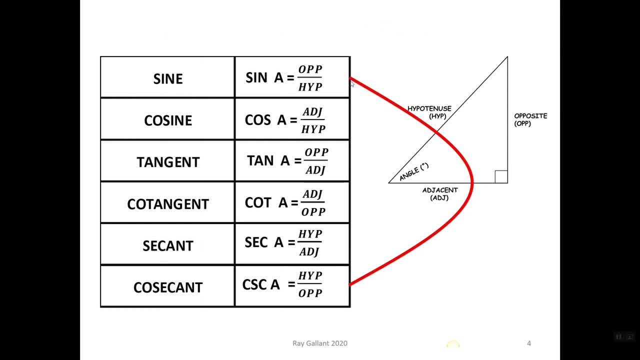 If we take a look, some of these have relationships. Okay, so our opposite and hypotenuse for our sine and our cosecant. hypotenuse and opposite is just the inverse of sine. So when we type on our calculator, we're not going to find a cosecant button. What we'll find is a sine button. 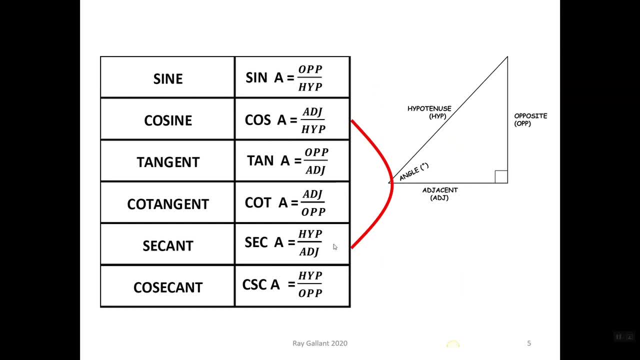 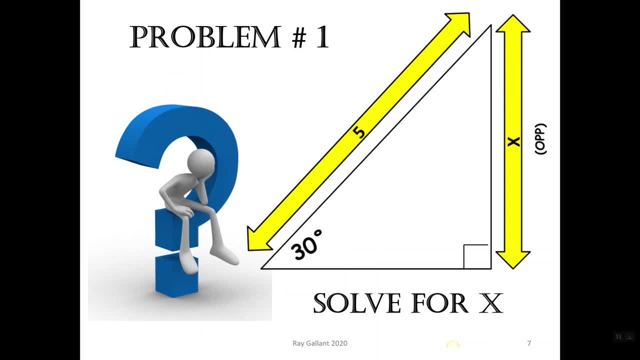 Same with cos and secant: they're just inverted. And the same with tan and cotangent. Okay, problem number one: What we have is we have one side here that's five inches, and what we want to know is x. We also have a 30 degree angle, So if our angle's here, 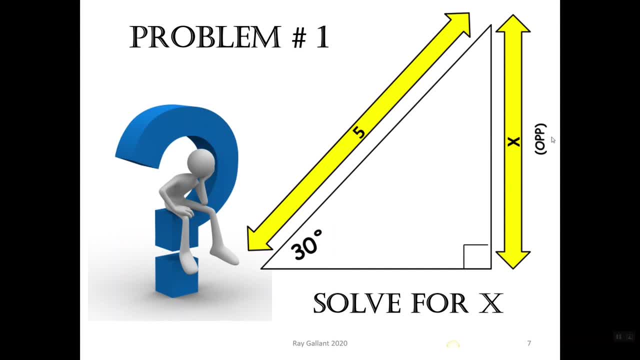 this length here is called the opposite side. The longest part of the triangle is called the hypotenuse. So what we have is a question. When we solve our questions, we want to solve for what's on top. So we're going to put our opposite on top. 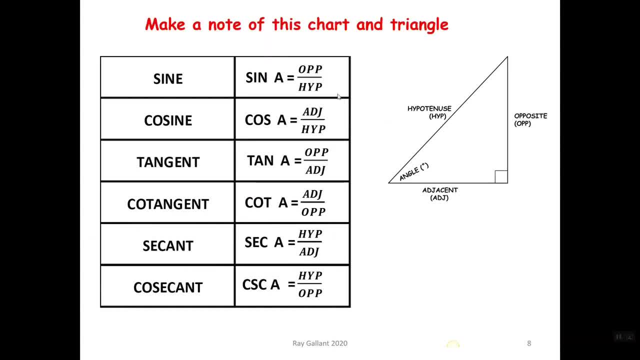 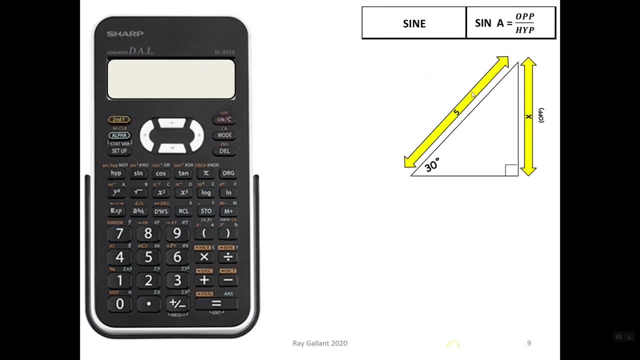 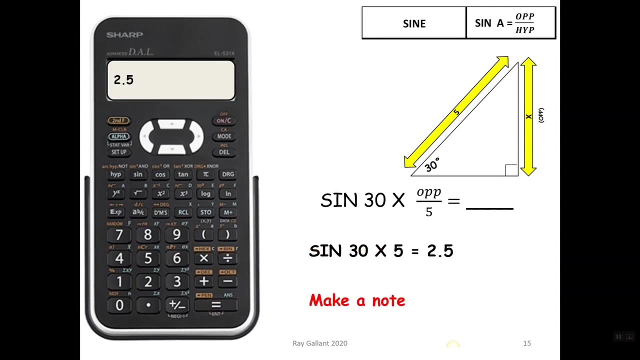 over our hypotenuse. So if we look opposite over hypotenuse is going to be sine. Then we turn around we say: okay, let's get out our calculator, follow along with me, We're going to type in sine. Then we're going to type in: 30 times 5 equals 2.5.. So therefore x equals 2.5 inches. So the opposite side. 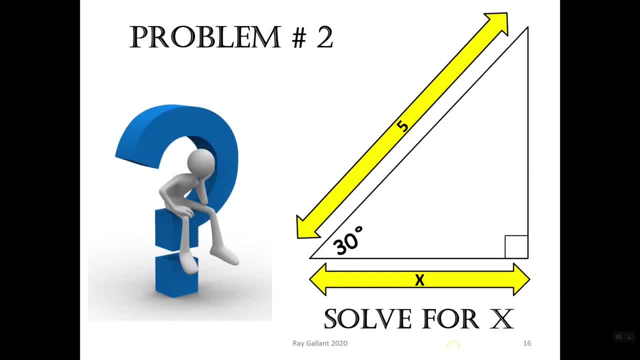 is two and a half inches long. Okay, problem number two. So now what we have is: we still have our length here, our largest side, which is called the hypotenuse. You're right Now, this one here, because the the angle is right here. what's this guy called? 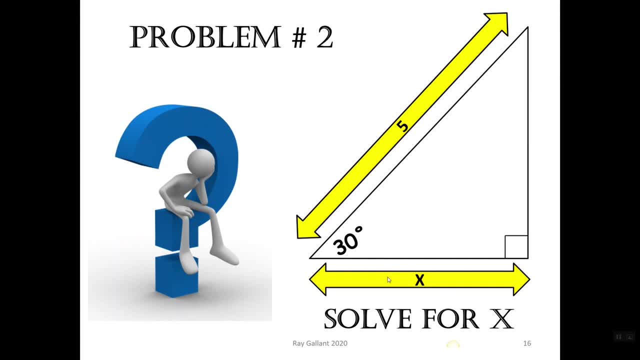 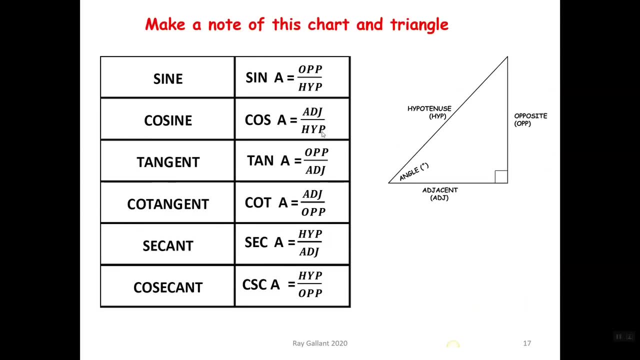 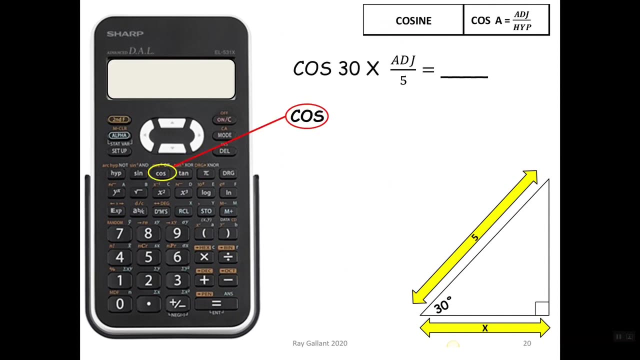 This is the adjacent. So what we want to find we're going to put on top. So it's going to be adjacent over hypotenuse. So adjacent over hypotenuse is cosine. Okay, we pull out our calculator again, We're going to type in: cos 30 times 5 equals 4.3301.. Therefore, x equals 4.331. 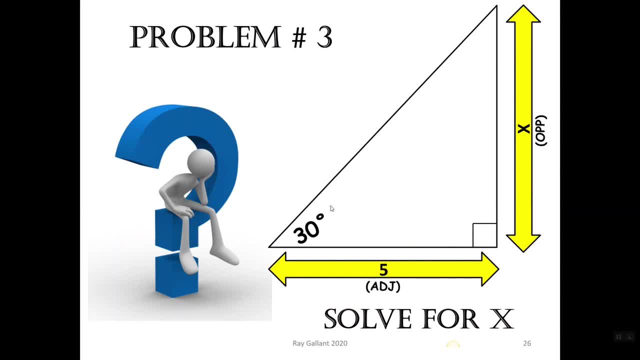 Problem number three: We have our 30 degree angle, We have one length and we have a second length. So what we want to find here is the opposite side, and what we have is the adjacent side. So what we're going to do is we're going to put the 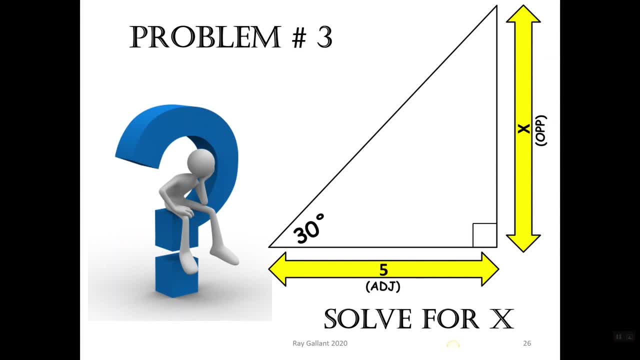 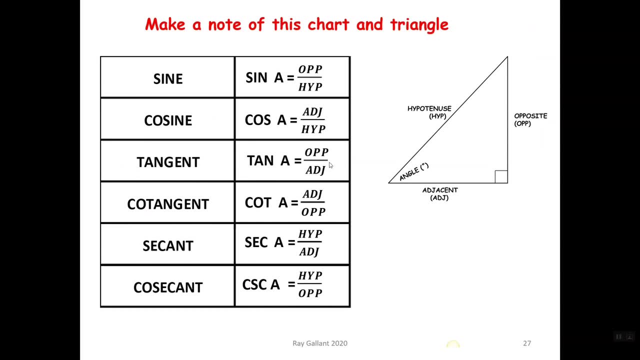 one we want to find on top, same as we did with all the other ones and all the ones we're going to do. So our opposite goes on top of our adjacent, Opposite over adjacent. So we're going to be using tan. 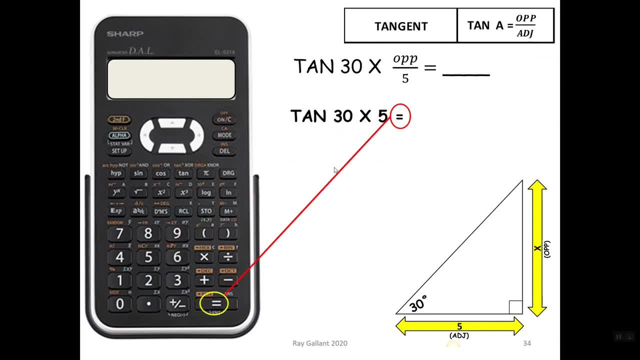 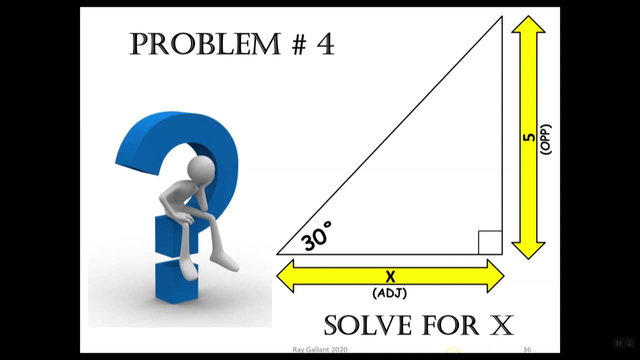 Tan, 30 times 5 equals 2.886.. That's not so difficult. now is it Problem number four. We're still solving for x. Now this problem seems very familiar because we just did one that looks very familiar to this. 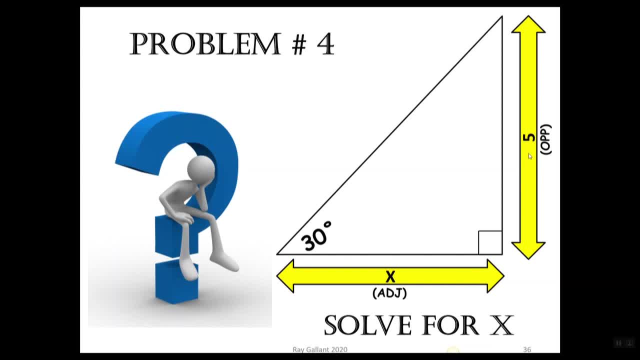 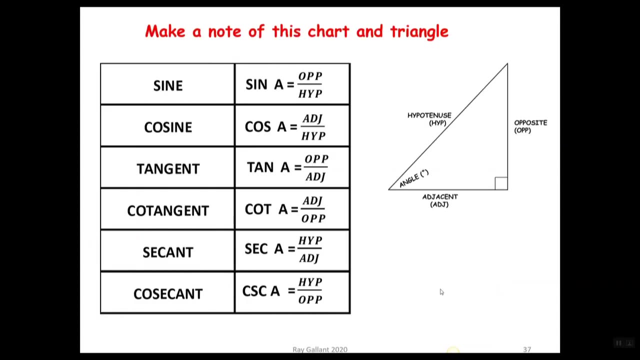 On our last problem, we were solving for the opposite and we had the adjacent. Now, this time we have the opposite and we're trying to find the adjacent. okay, so what we want to find, we want to put on top. so we're going to say adjacent over opposite. 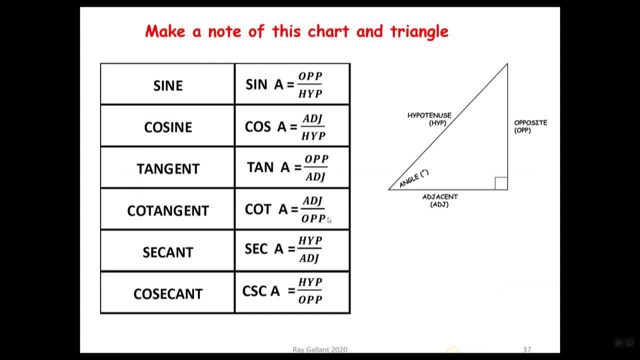 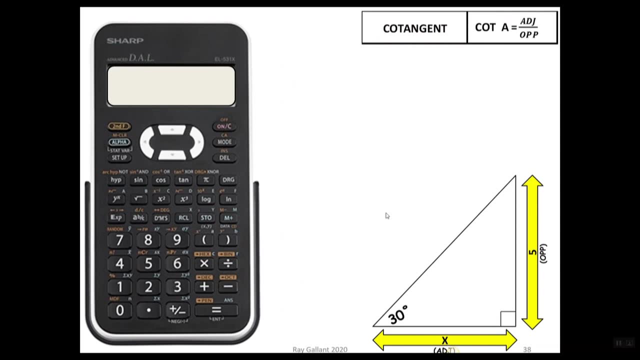 adjacent over opposite. do we remember the relationship that we had between tan and cotangent? tan is just, or sorry, cotangent is just inversed of the tangent. so how do we type this into our calculator? we're going to type in: tan 30 equals second function 1 over. so that's going to 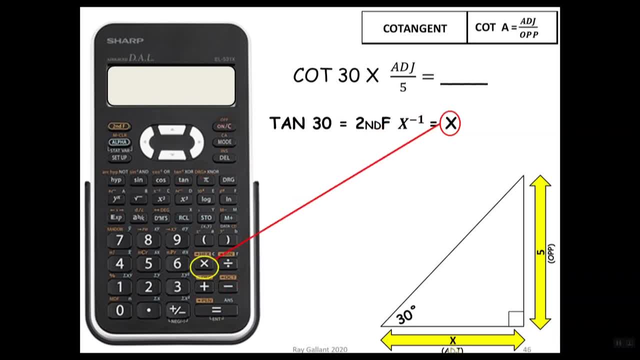 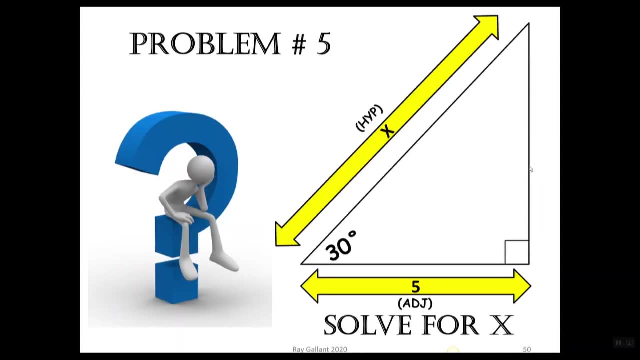 inverse: the tan equals times 5, equals eight point six, six, zero, two. so therefore the adjacent length here is eight point six, six, two or zero two. problem number five: so what we have is: we have the five inches here, but we want to find out what X is. so therefore we don't know this length. 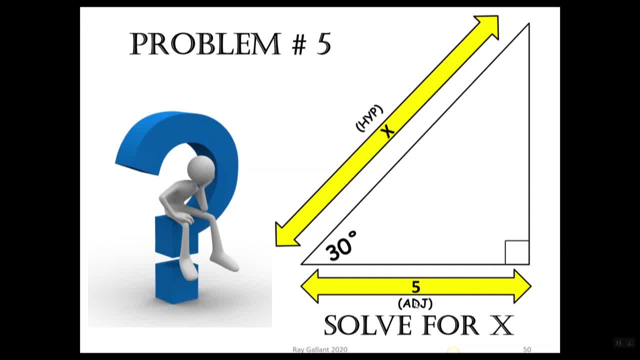 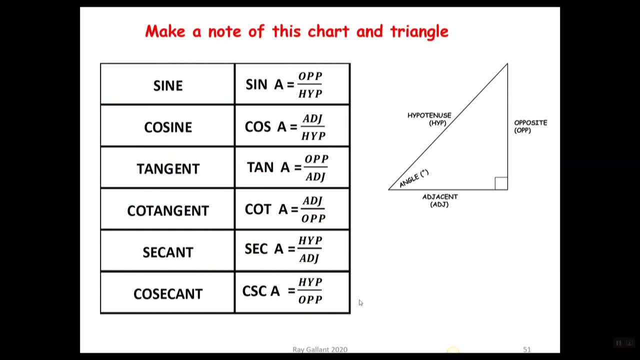 here's our angle. so what we want to find, we're going to put on top. so we're going to put hypotenuse over adjacent. let's go to our chart here: hypotenuse- hypotenuse over adjacent is going to be secant if we remember our relationships. cosine and secant have a relationship to each. 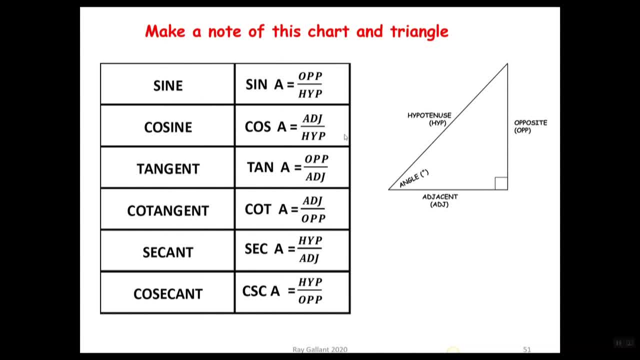 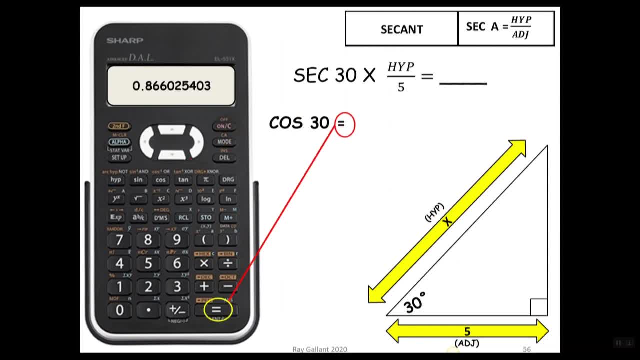 other secant is the inverse of cosine. okay, so we're going to type in: cos 30 equals second function 1 over. so we're going to inverse that amount. now times five equals five point seven seven four. therefore the hypotenuse is five point seven seven four. now let's take a break for a second here. 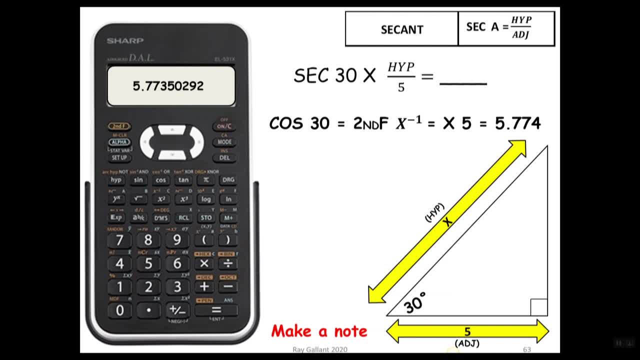 sometimes your calculator lies to you. we can agree with that. sometimes it does. what if I accidentally press the button that I wasn't supposed to press or I made a mistake typing a button in one of the ways that you can instantly tell that your your answer is incorrect if this length here is less than this length. 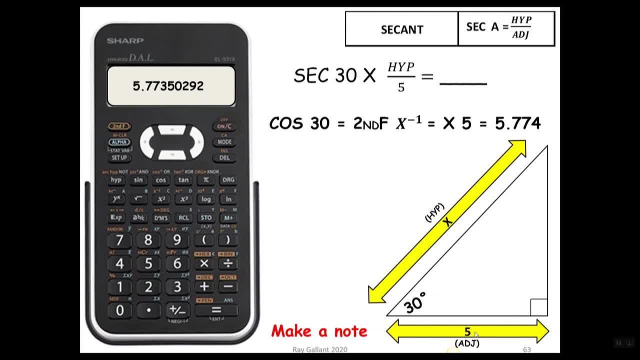 if this was four point seven, seven, and this length here is five. you know there's a mistake right away, because the hypotenuse is the longest side, so it has to be larger. so if you're getting a smaller number, don't trust your calculator. start over, redo it. 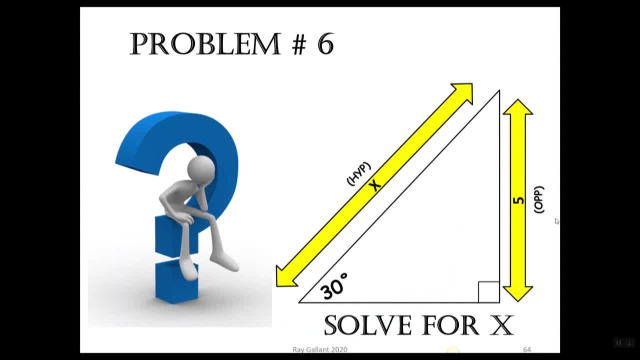 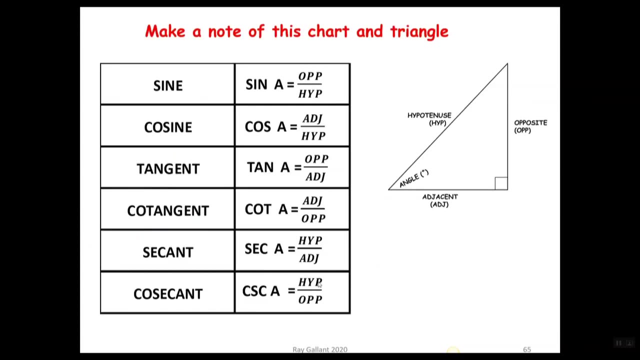 again, problem number six. okay, so what we have here is we have the opposite length and we want to find our hypotenuse. okay, let's go to our chart. so we're gonna say: hypotenuse over opposite, hypotenuse over opposite. okay, cosecant, which is the 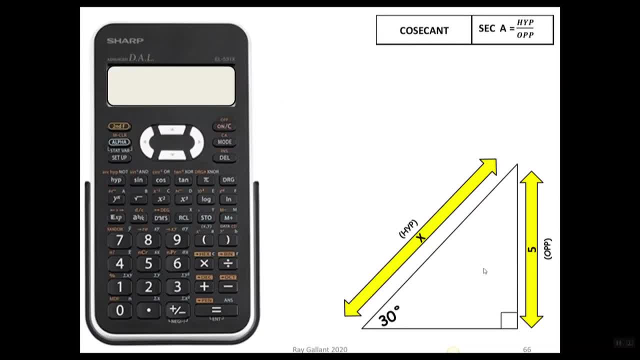 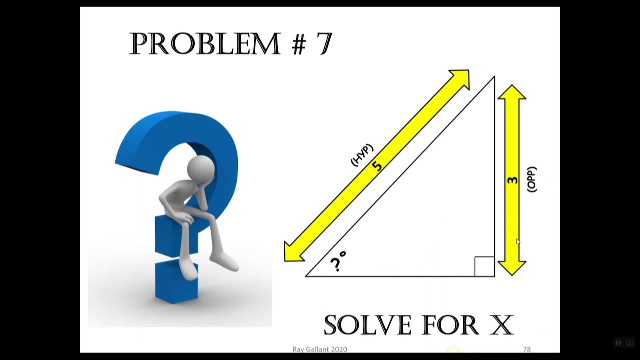 inverse of sine. okay, sine 30 equals second function: 1 over equals times 5 equals 10. problem number seven: problem number seven: okay, here's a tricky one. I have the length of my opposite, I have the length of my hypotenuse, but wait a second, I don't have an angle. 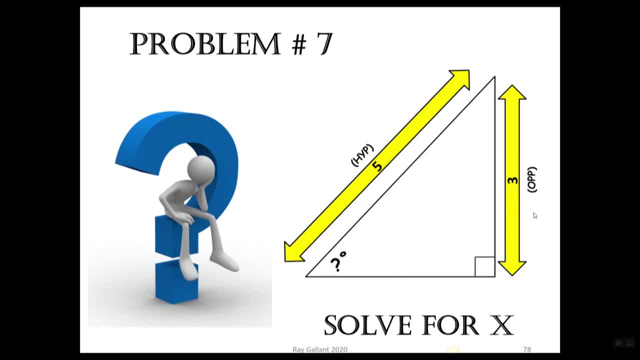 okay. so we know that we're going to be using opposite and hypotenuse in this one. when we solve, we're going to be using the upper three of our chart. here we're well, we're just going to be use finding angles. we only want to find. 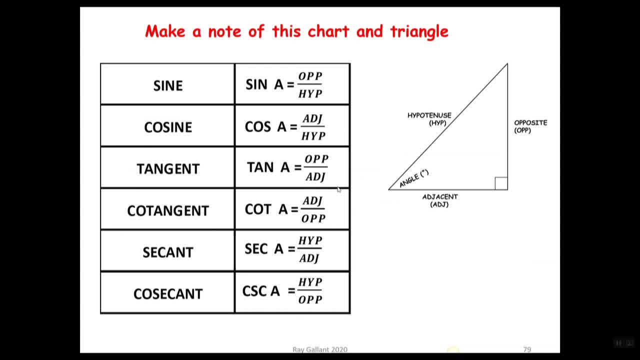 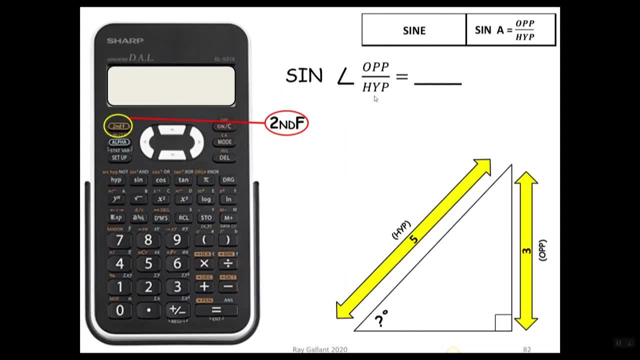 these three. We don't want to use these ones because we don't want the inverse. okay, So we're going to use opposite over hypotenuse. So we're going to go second function sine, and you're going to type your bracket in: 3 divided by 5, bracket equals, and then 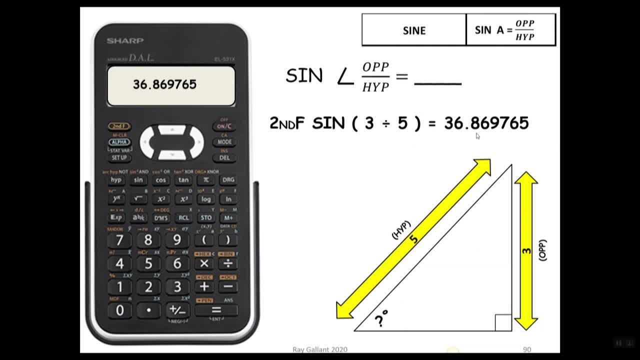 you're going to come up with 36.869765.. Second function: DMS: 36,, 52 minutes and 12 seconds. Now, if you're doing, if this was a metric question, it would stay as a decimal, Okay. 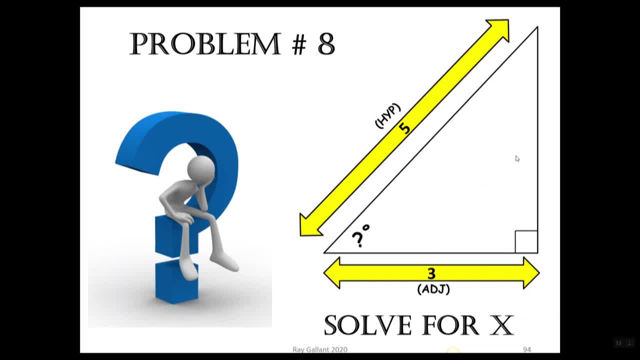 let's try another one, Problem number 8.. Okay, so we have the hypotenuse and we have the adjacent, but we don't have our angle. So hypotenuse, adjacent, adjacent, hypotenuse. we know that this is going to be cosine. Okay, 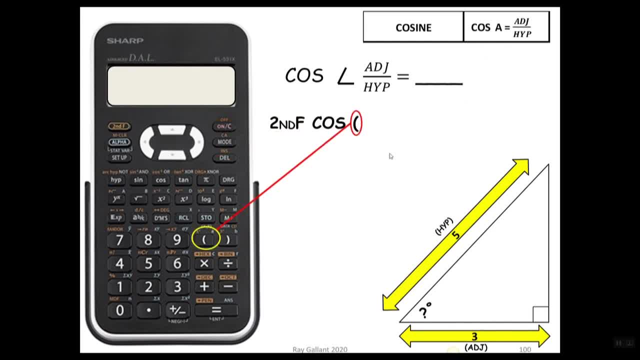 so we're going to go second function: cos, bracket 3, divided by 5, bracket equals 53.1301.. So we're going to second function this: DMS: degrees, minutes, seconds, and it comes out with 53 minute or 53 degrees. 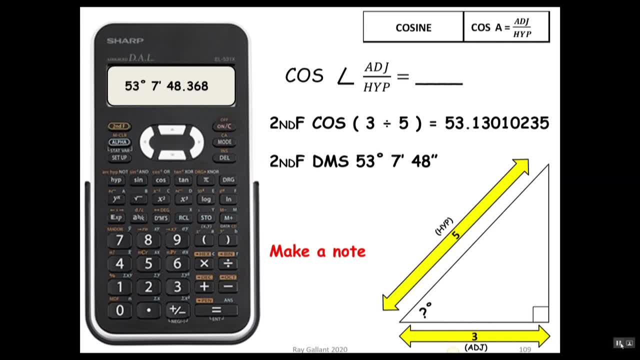 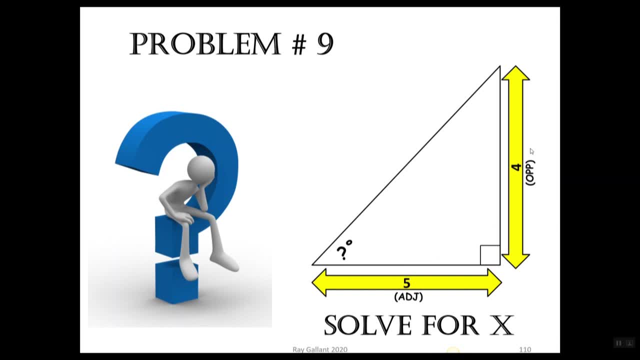 7 minutes and 48 seconds. Problem number 9, the last problem. Okay, so what we have here is we have the opposite and we have the adjacent. We want to find our angle. So, opposite, adjacent, We go to our chart. 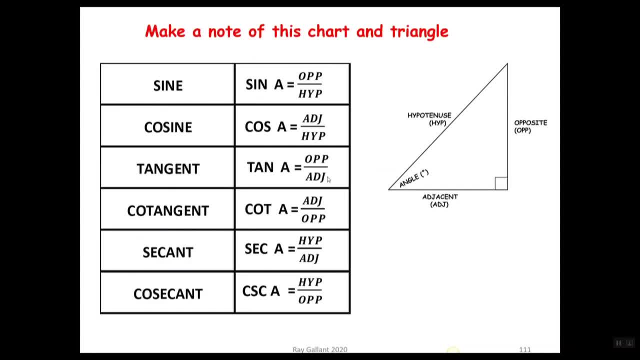 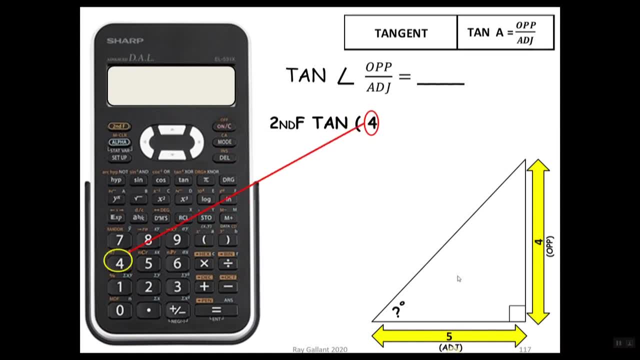 here opposite adjacent. So we're going to be using tan. Second function: tan, bracket 4, divided by 5, bracket equals 38 degrees 0.65.. Second function: DMS: 38 degrees, 39 minutes. 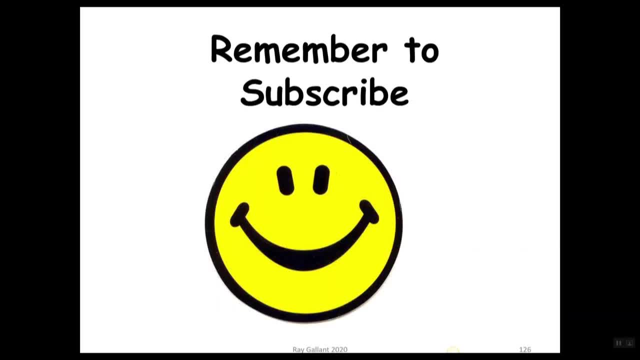 and 35 seconds. Don't forget to subscribe. I hope that this video has given you a broader understanding of trigonometry. Keep in mind, there's only 9 possible solutions to most trigonometry questions. There's also a lot more in here. 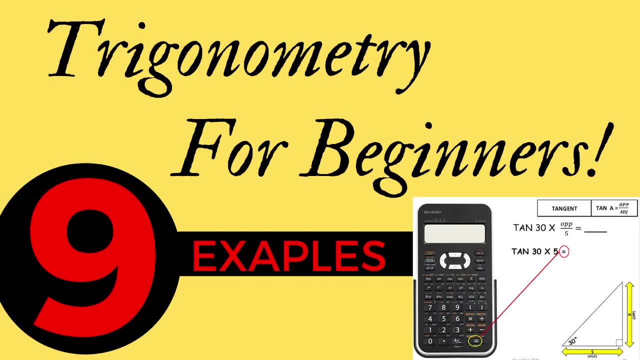 Thank You, See ya more trigonometry questions and answers on my youtube channel shop and math. if you enjoyed the video, please like and subscribe. it's free and it'll help me out. all you have to do is click on the icon on my face and I'll do the rest.